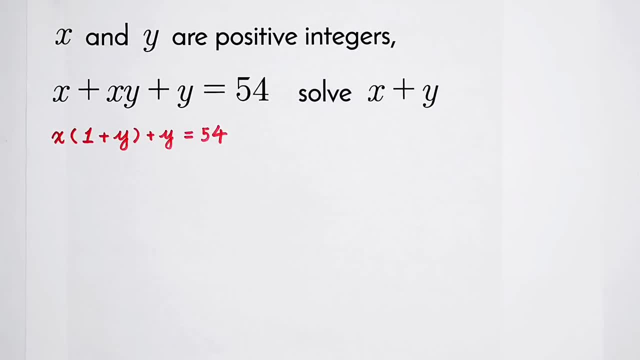 But we can try If we want to find the factor, if we want to take out something, and we have to take out 1 plus y when we can continue to factor on it. But now here is just a y left. So now I'm going to add a 1 on the left-hand side. 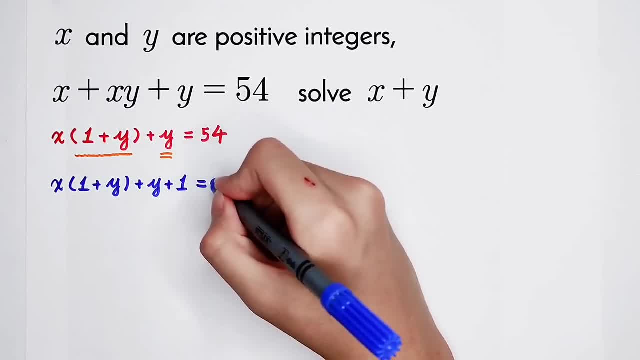 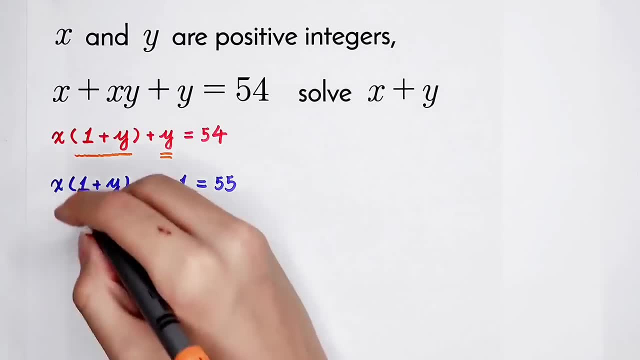 And also on the right-hand side, 54 plus 1 is 55.. I think this number is very good. It's a good-looking number, isn't it? So now, 1 plus y, y plus 1, take it out, Then you have good luck. 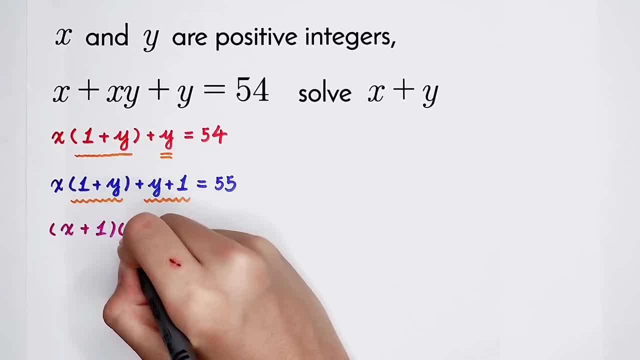 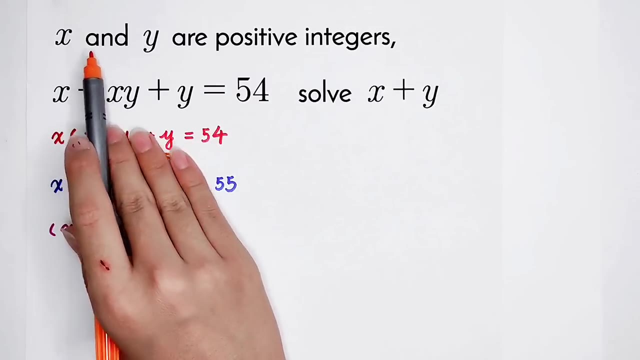 x plus 1, and then times y plus 1.. It is 55.. 55. We have to have a look at this problem again. The knowing It says x and y are positive integers. So because x and y are both positive integers, 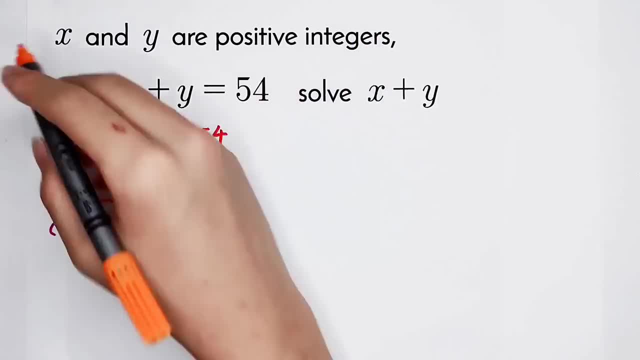 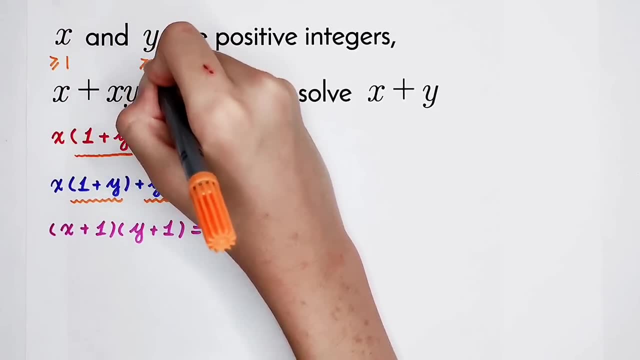 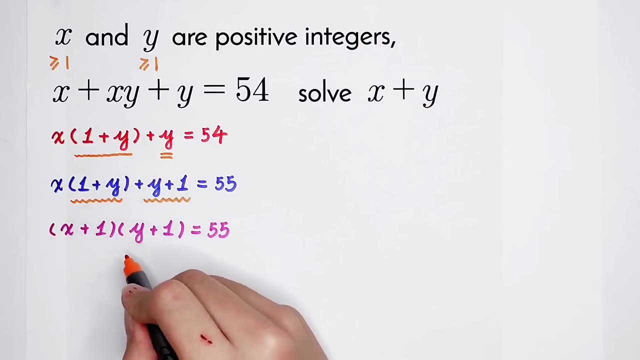 then I can get x and y. they are integers and they both. they are both greater or equal to y, Because x and y are positive integers, So x plus 1, and then y plus 1, they are also positive integers. 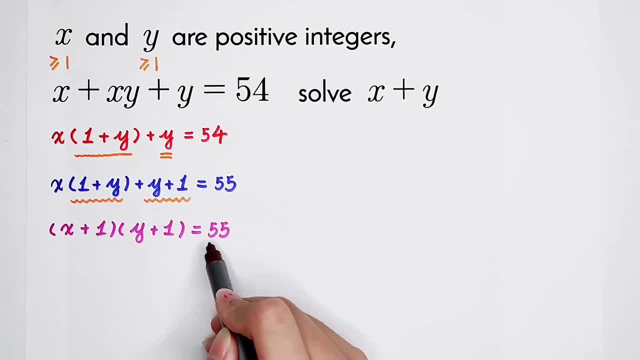 Aren't they? Now we find the factor of 55.. Because 55, it can be written as 1 times 55, itself 1 times itself and itself times 1.. And then it can also be written as 11 times 55.. 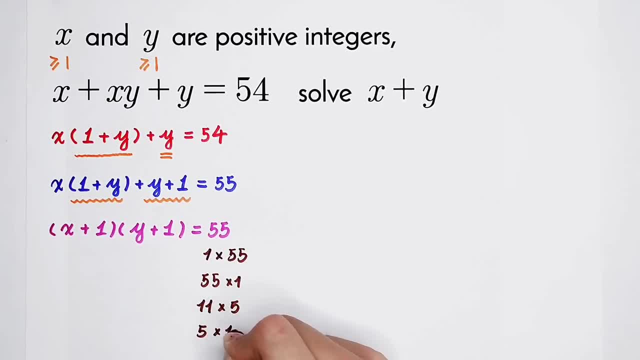 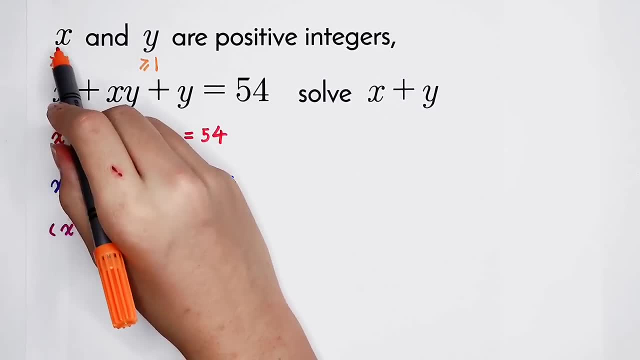 And 5, then multiplies by 11.. There are 4 cases, But are they correct? From here? x and y, they are both integers and they have to be. they both have to be greater or equal to 1.. 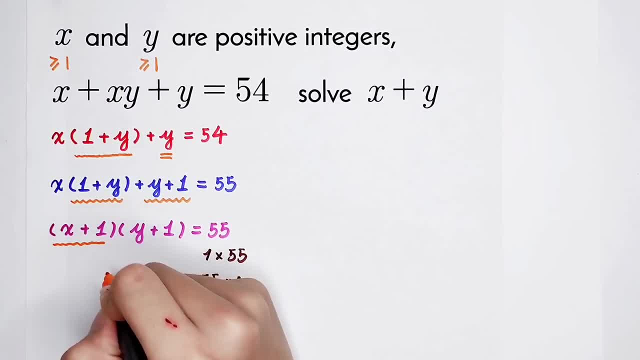 And then x plus y. it is also an integer and it has to be greater or equal to 2.. y plus 1.. The same case, So 1 times 55,. cancel 55,, then times 1,.